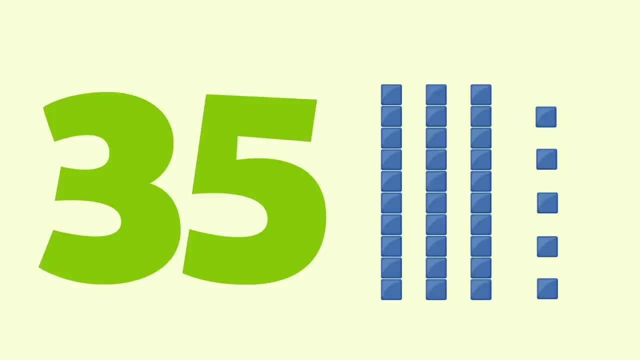 in the ones place always equals itself. In our number 35, the five is in the ones place. Its value is just that five. It is represented by the five ones cubes. The next place over is the tens place. The number in the tens place is always ten times the value, the number. 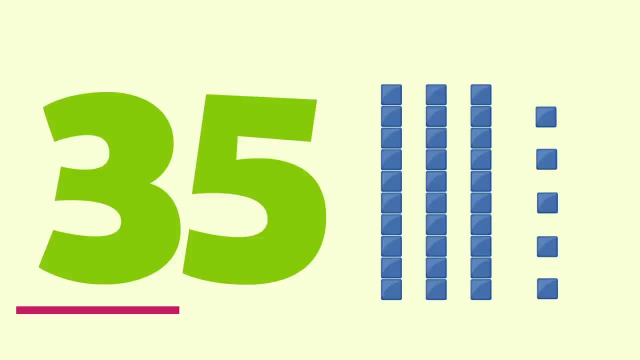 shown. It's like counting by tens to the number. you see In our number 35,, the three is in the tens place. We can find its value by counting by tens three times. Let's try it: Ten, twenty, thirty. The value of the three is thirty. Another trick you can remember is to just 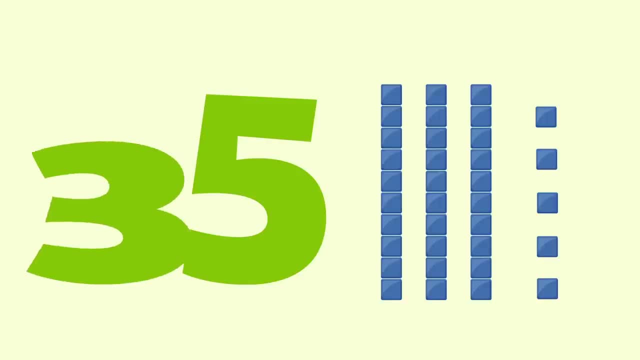 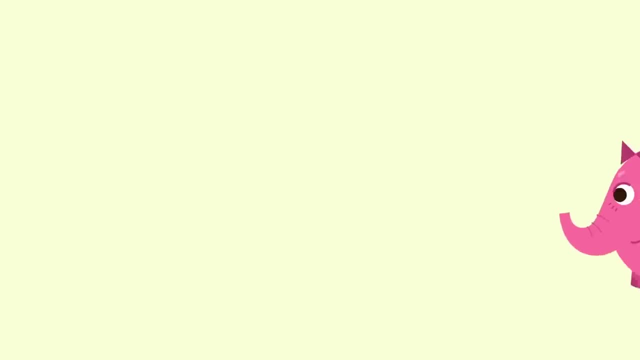 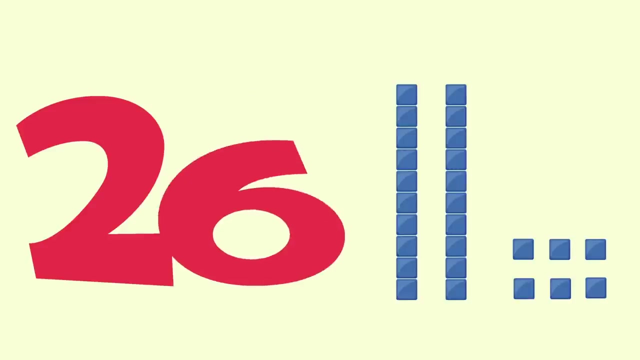 put a zero at the end of the number, The three in thirty-five is represented by the three tens blocks, which equals thirty In the number twenty-six, the six is in the ones place and the two is in the tens place. The six is worth just six, which is represented by six cubes. 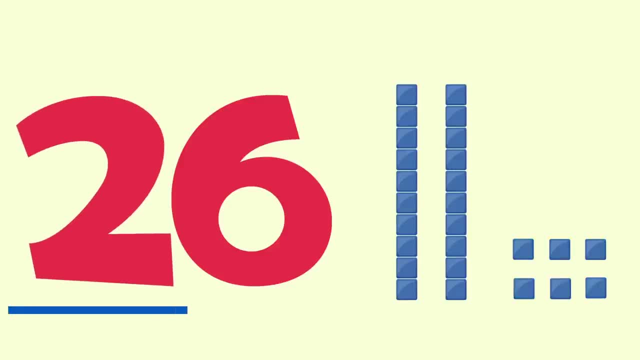 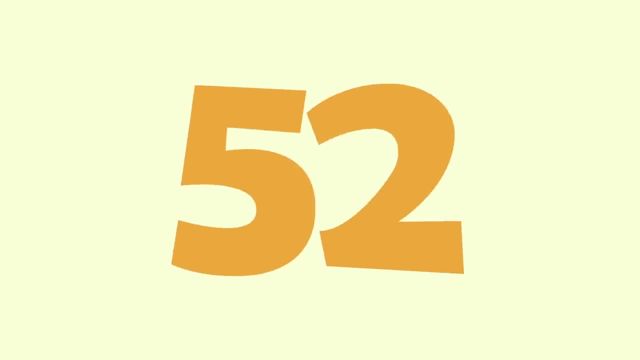 The two is worth twenty because it is in the tens place and is represented by the two long tens blocks. You can count by tens using the base ten blocks or just count in your head Ten, twenty. I'll leave you with a challenge. Can you tell the value of the digits in the 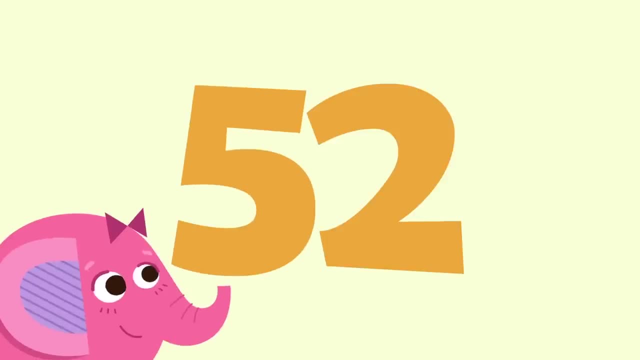 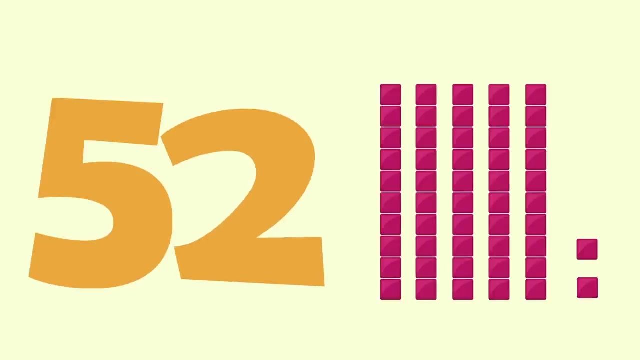 number fifty-two. What is the value of the five? What is the value of the two? I'll give you some time to think, But if you need more time, you can pause the video and answer when you're ready. Okay, here's the answer. The two is in the ones place, so it's just worth two. The five: 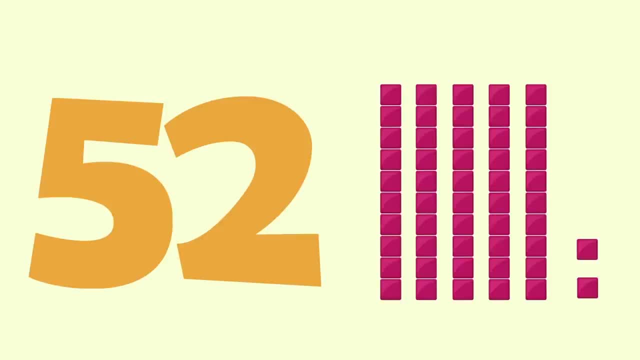 is in the tens place, so we'll have to count by tens. five times Ten, twenty, thirty, forty, fifty. The value of the five is fifty. Remember to look at the place the digit is in before you decide the value of that number. Thanks for watching boys and girls. See you next time.